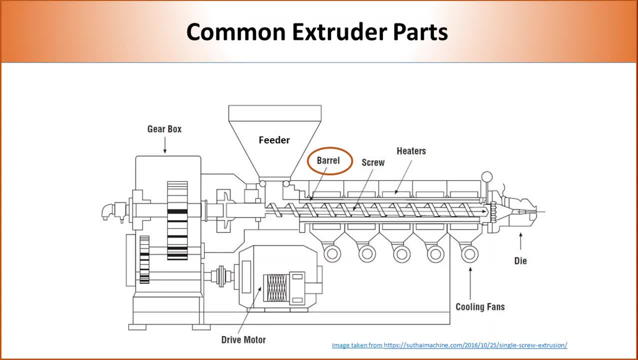 extruder. The inner layer of barrel is specifically treated to eliminate any reaction with polymer at high temperature. Heaters are mounted on the barrel to melt the polymer and keep it at desired temperature during extrusion. Several heaters are used to separately hotter the top layer of the 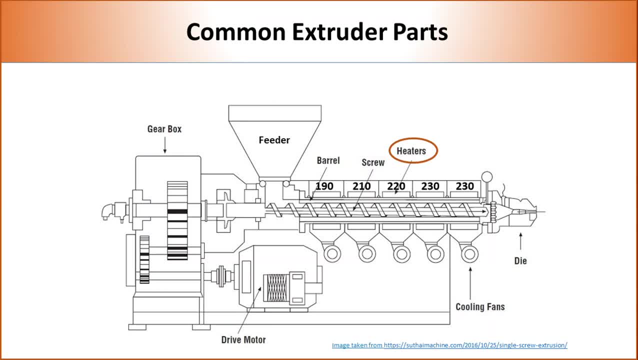 barrel. One of the interesting benefits of single-switch儿 extruders is the ability separately control the temperature at different zone. mostly, extrusion is performed at 50 degrees c higher temperature than the melting point of polymer. the temperature profile of polypropylene. 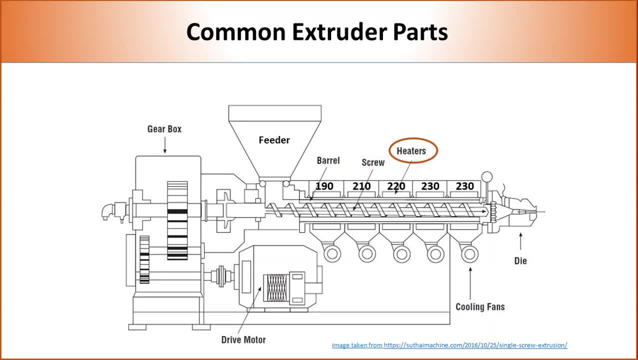 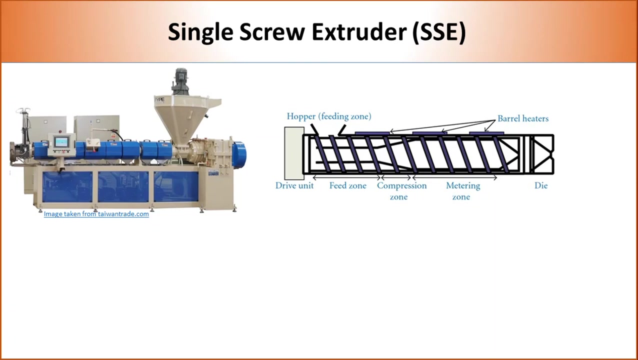 is shown in the picture, which has a melting temperature of 165 degrees c. and finally, all extruders contain motor and gearbox to generate motion and transfer motion from motor to screw. every component of the extruder influences the mixing quality and efficiency. as mentioned previously, single screw extruders contain one screw, the screw mostly. 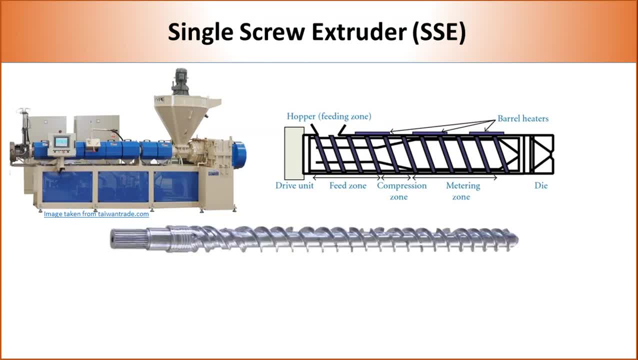 is a single metallic shaft containing flights to guide the polymer inside the barrel. most screw contains three distinct sections for First section is called feed section. In this part flight depth is high so that more amount of plastic beads can fit in. As plastic is fed through the hopper, it melts and move forward due to back pressure. 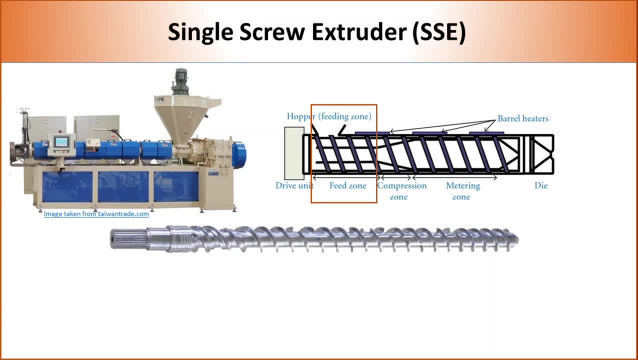 Back pressure is the most important factor which controls flow of polymer inside single screw extruder. Second zone is called compression. In this section the flight depth gradually decreases. It allows polymer melt to get compressed and release any volatile material which can be harmful for the polymer. 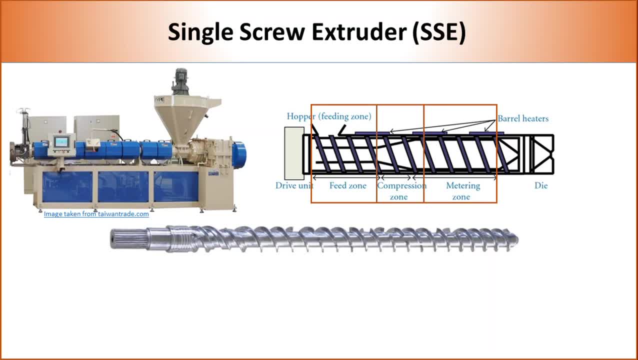 The third zone is called metering. In this section, flight depth is very narrow, which creates high shear and thus help additive to disperse in the polymer matrix. It is important to know that the relative length of each zone depends on the polymer's melting behavior and the viscosity of polymer melt. 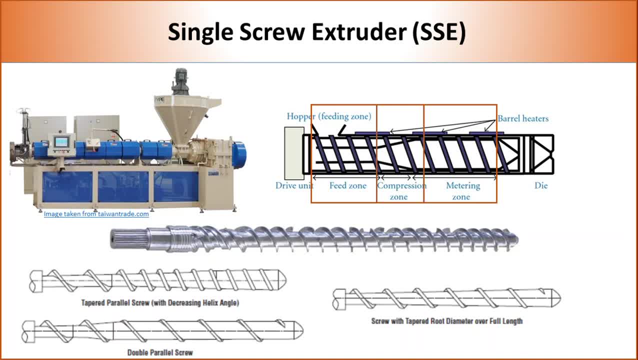 If polymer are difficult to melt, it needs longer feed zone, But if polymer possess very low melt viscosity, then we need to use small feed zone and long compression zone. Therefore, This type of screw design is available in the market, as shown in the picture. 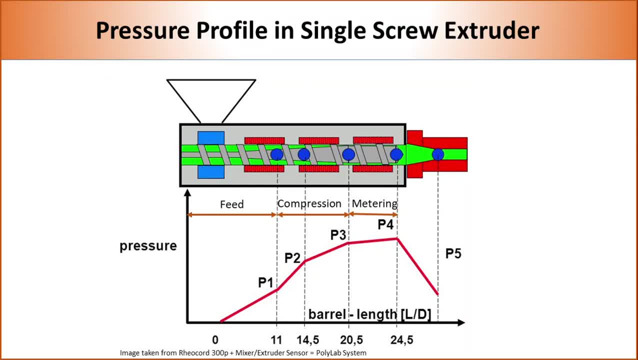 Pressure inside a single screw extruder is shown here. We can see that pressure gradually increases from feed zone to metering zone. The increase in pressure is related to decrease in flight depth. The pressure also reflects the amount of shear applied in each of the parts. 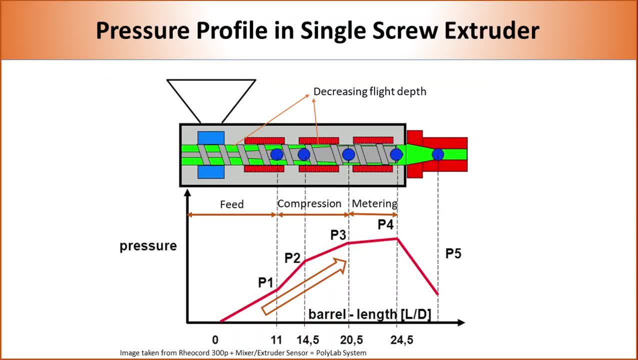 This type of screw design is available in the market as shown in the picture. Pressure inside a single screw extruder is shown here in each zone. As polymers are always under pressure inside the barrel, we cannot put vent in single screw extruder because polymer melt will shoot out from. 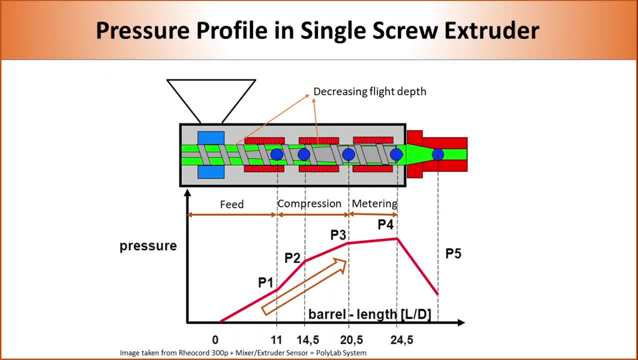 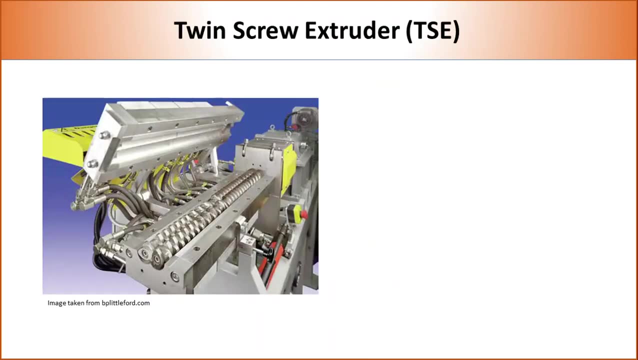 the vent. Recent development in a screw design have allowed putting vent in the single screw extruder, but it is still not widely adapted. Now coming to twin screw extruder. Twin screw is much more versatile than single screw extruders. Presence of two screws allows several variations in terms of 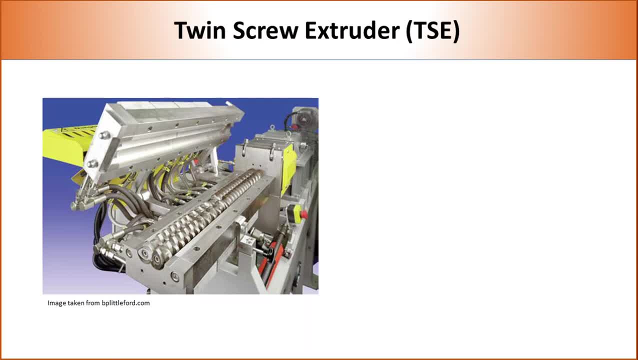 rotation, position and type. Therefore, there are several types of twin screw exist in market Based on rotation. twin screw can be classified into co-rotating and counter-rotating. In case of co-rotating, both screw moves in the same direction, whereas in counter-rotating screw rotates in opposite direction. 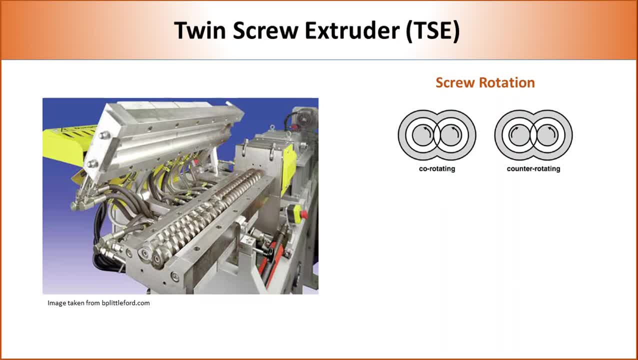 For plastic compounding, co-rotating twin screw extruders are mostly used. In term of position, twin screw can be classified into intermissing and non-intermissing. In intermissing, two screws are positioned very close to each other so that flights of one screw enters in the 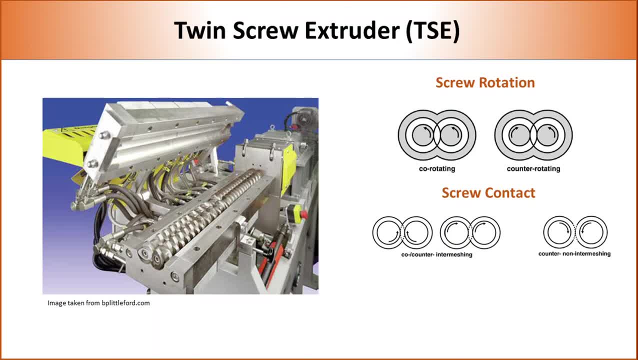 flight depth of other screw. Arrangement of screw in this way allows self wiping of screws and better transfer of polymer melt from one screw to another screw. In non-intermissing screws are positioned far apart so that flights do not enters in each other space. 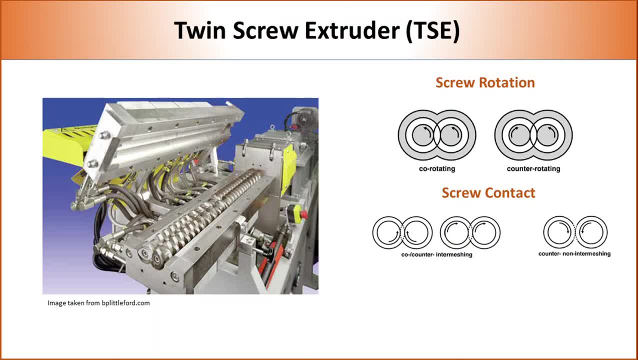 These types of two screw are not suitable for co-rotating In. non-intermissing screws are positioned far apart so that flights do not enters in each other space types of twin screw are used for high throughput compounding. Twin screw can also be classified by the screw types, like single shaft or modular. 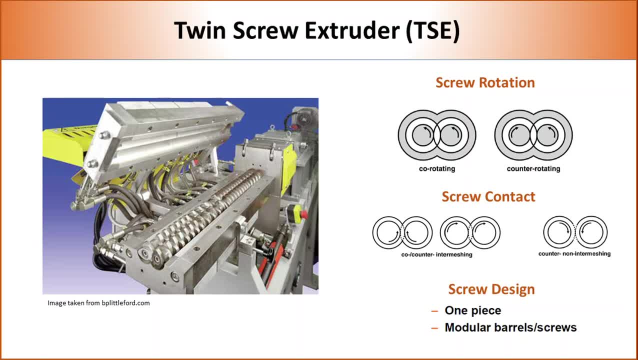 Single shaft screws are very similar to single screw extruder. Single shaft screws provide option to achieve very high shear. but to process different types of polymer and additives whole screw needs to be changed. The modular screw consists of individual elements arranged on a shaft. As elements can be arranged in a wide number of ways, the screw design can be extremely. 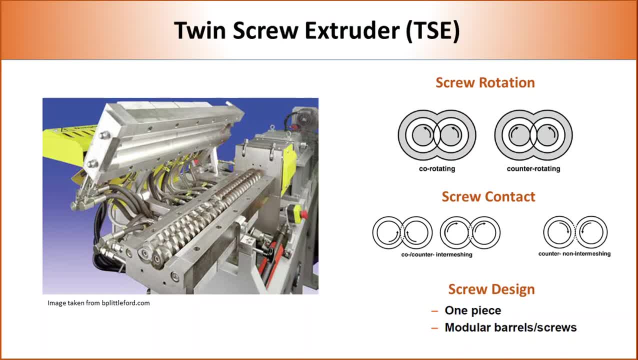 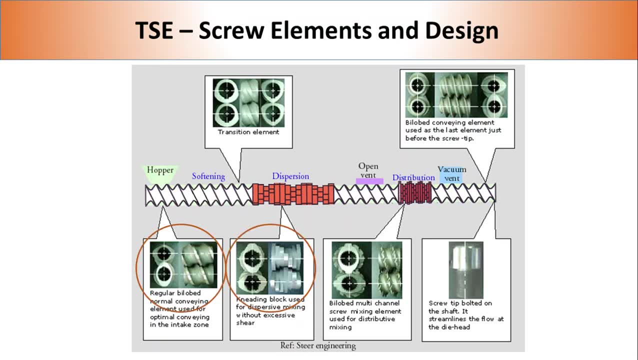 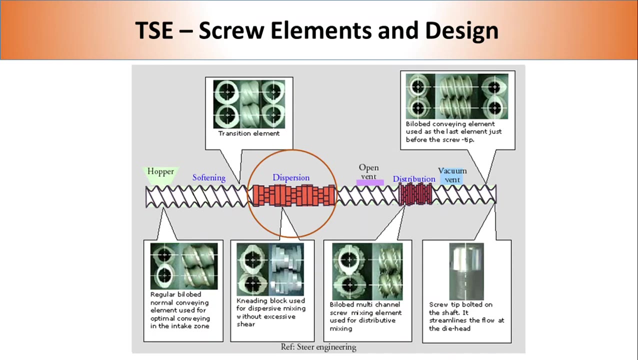 versatile. Most common elements in a twin screw extruders are conveying element, kneading block and flow restrictor. Number and location of these elements can be easily changed. thus provides huge amount of flexibility during compounding. Kneading blocks provides high amount of shear, thus help to achieve excellent dispersion. 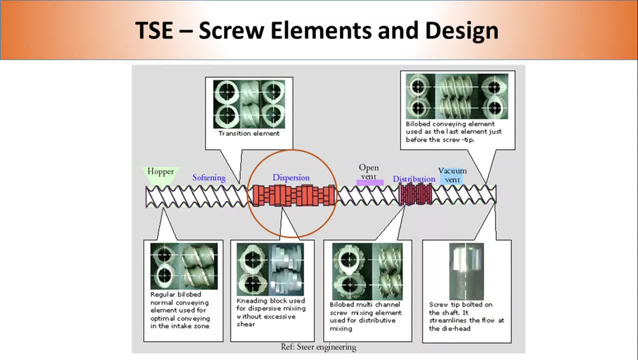 of additives. However, if the polymer is sensitive to extensional flow, having kneading block can be a problem. Flow restrictors reverses the flow of polymer melt, thus allows additives to mix properly in the polymer matrix, Depending upon the difficulty of dispersion. a typical screw of twin screw extruder will. 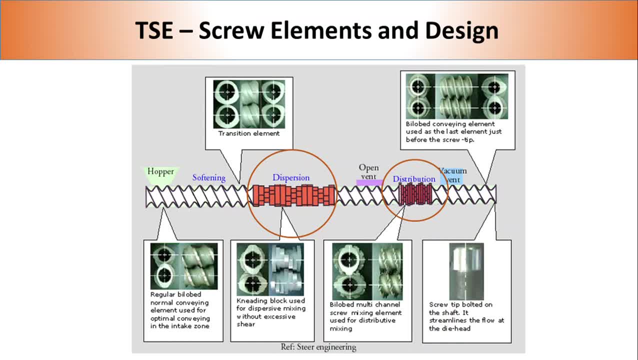 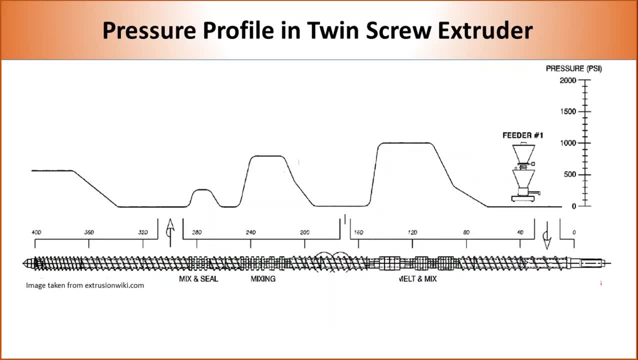 consist of one or more section of kneading and flow restrictor blocks, as shown in the image. Presence of various types of elements in the screw also leads to different pressure level inside the barrel. Here we can see that after feeding, Pressure increases as polymer melt moves forward. 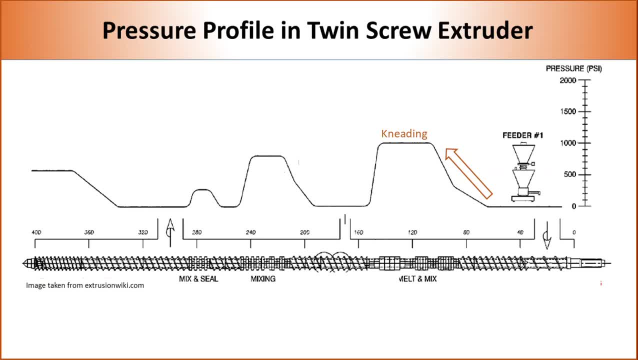 Highest pressure is developed at kneading block. The pressure again drops as we move to conveying element from the kneading element. We can see here that depending upon the offset angle of kneading block, different amount of pressure is developed at different kneading block section and almost no pressure is developed. 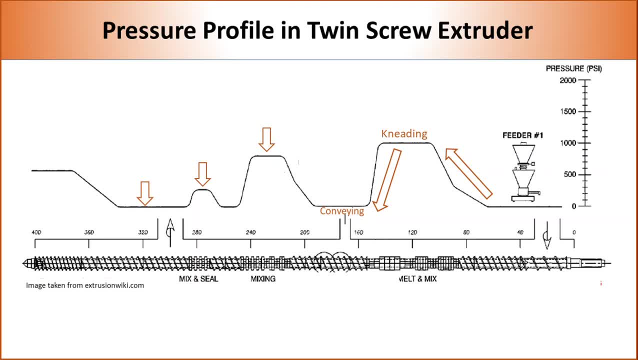 at the conveying section. Presence of sections with zero pressure allows manufacturers to put extra feeder and vent at different part of the machine. The ability of a twin screw extruder to provide opportunity to have multiple feeders and vents significantly enhances its mixing ability and efficiency. 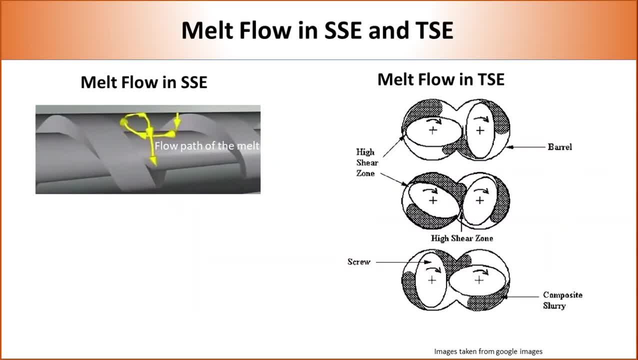 Conclusion: Actually, the presence of two screws significantly changes how polymer is processed in twin screw compared to single screw extruders. the most important difference is: in single screw extruder, polymer melt flows passively due to back pressure. on the other hand, in twin screw extruder, there 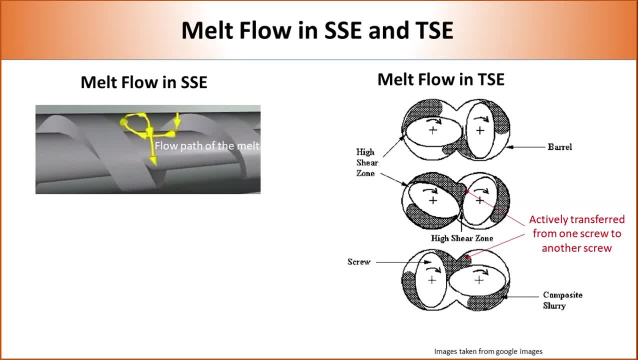 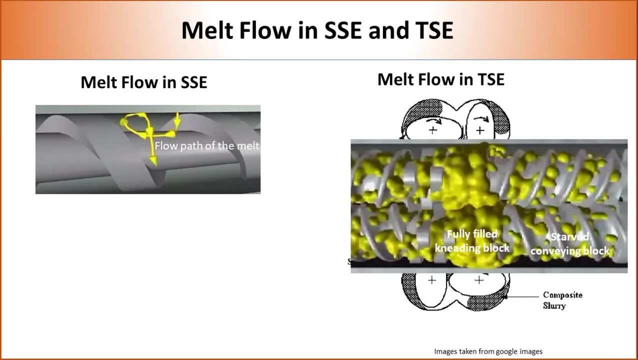 is active flow of polymer melt, since polymer melts are actively transferred from one screw to another screw. the active flow of polymer melt provides two very important benefits. first, twin screw extruder can run in a starved mode, which means it is not necessary to completely fill twin screw to move. 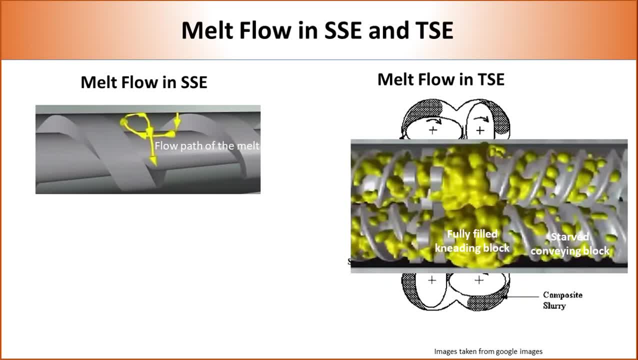 material forward. but in case of single screw extruder it is important to flood fade, otherwise polymer melt will not move forward. as twin screws are a starved fade, there is almost no pressure in conveying zone. another benefit of active melt transfer is that we can control how materials can. 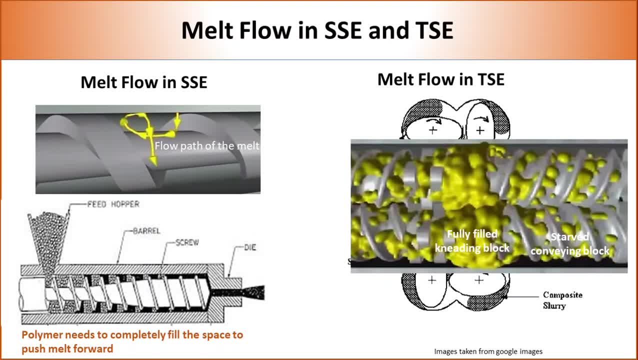 flow inside the barrel and how long it could stay in a specific segment of the screw. thereby, mixing efficiency can be optimized. overall, it can be said that extremely good mixing efficiency of twin screw extruder can be attributed to presence of high shear elements, vents and active material flows.